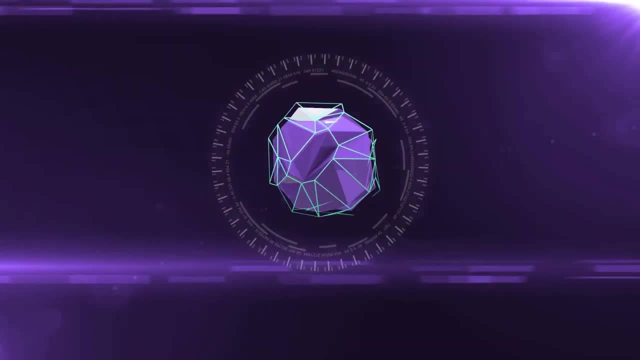 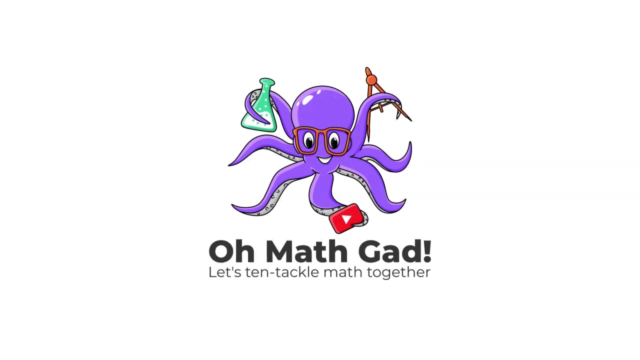 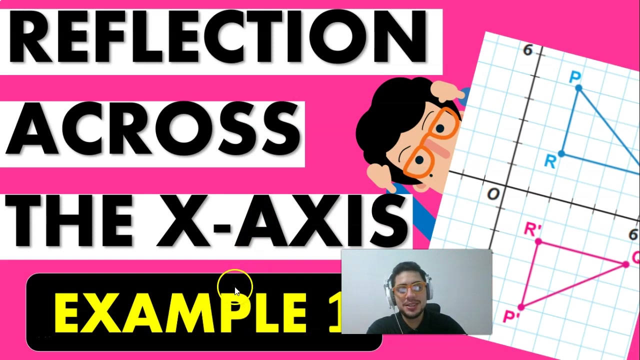 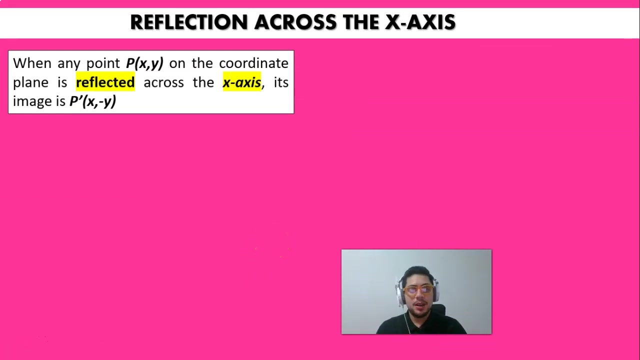 Hello guys, welcome to today's video in which we're going to be learning how to make a reflection across the x-axis. So let's begin, Okay, guys. so when any point P with coordinates x, y on the coordinate plane is reflected across the x-axis, it is very important to remember. 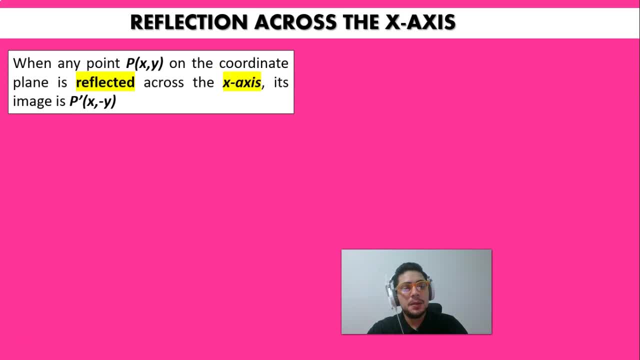 that the image, the resulting image, is going to be the same coordinate of x, but the y coordinate is going to be the opposite of what it was right. So we have to take this into account whenever we're reflecting any type of figure. So if the figure has five, 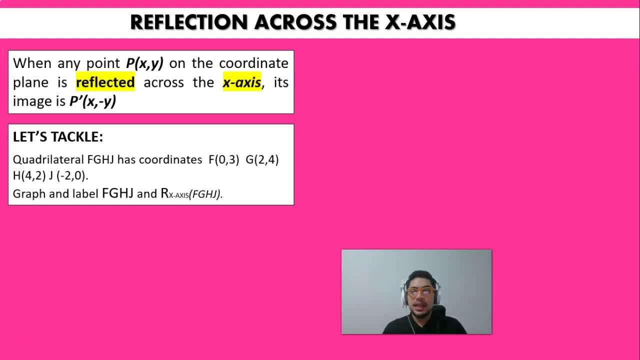 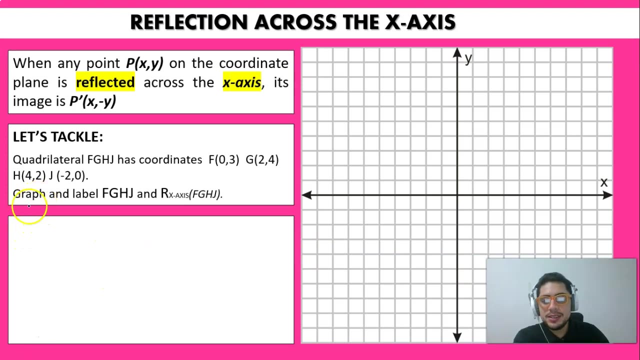 vertices, and it's going to be reflected over the x-axis, like the one we're going to be doing right here. the same case applies to the y's of every single point, right? So let's tackle it, guys, and let's make that graph. Okay, guys. so in this case we have f, which. 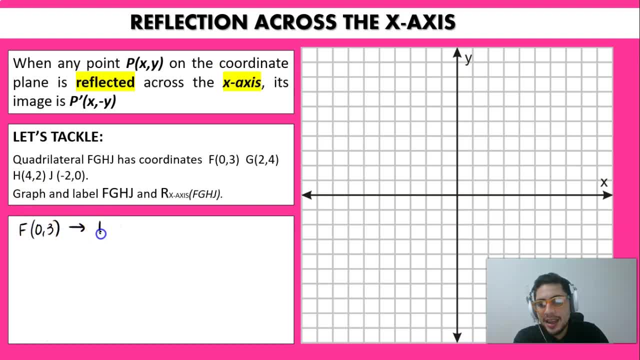 is 0,3.. So f tick mark is going to have the same value of x, but when it's rotated around the x-axis, like they're asking us to do, we're going to have a value of minus three. Then g is going to be two comma four. and now g tick mark is going to be two comma. 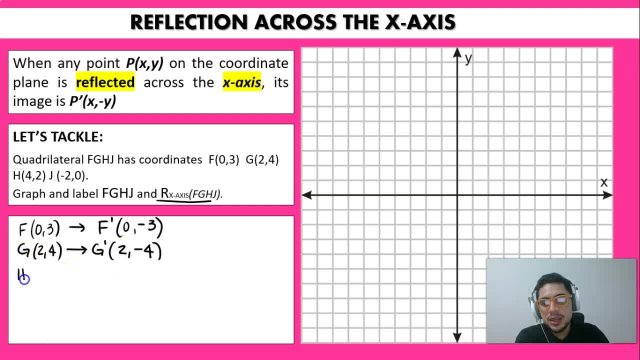 minus four. So as you can see, it's a pretty easy thing. We do the same thing with each and every one of the vertices. So h is four two. So h tick mark, or the reflected one across, is going to be four comma minus two, And then j, which is minus two comma zero, is. 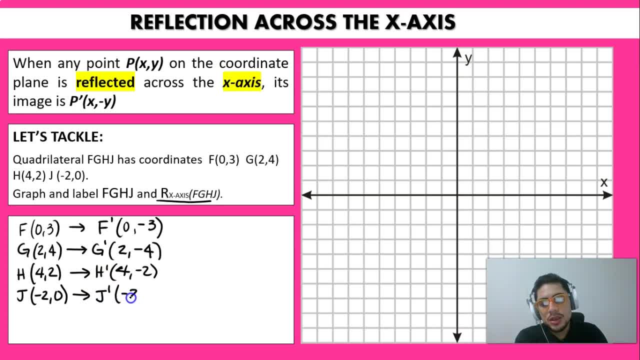 going to be j tick mark, which is minus two comma zero as well, because the opposite of zero is still zero. Okay, So let's try representing them on the coordinate plane. So let's first find the quadrilateral that they gave us, or the pre-image. 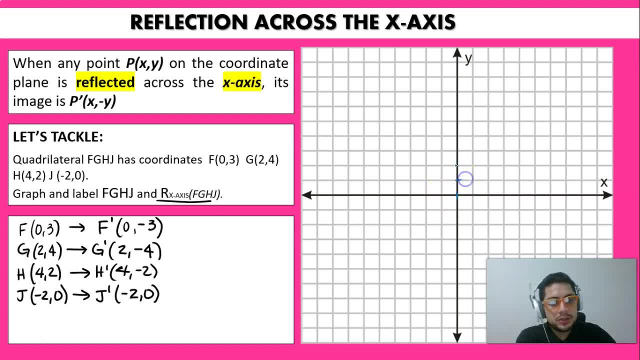 So h is zero comma three. So one, two, three. First one is going to be here And then we're going to have two comma four. So one, two, one, two, three, four. So this is f and. 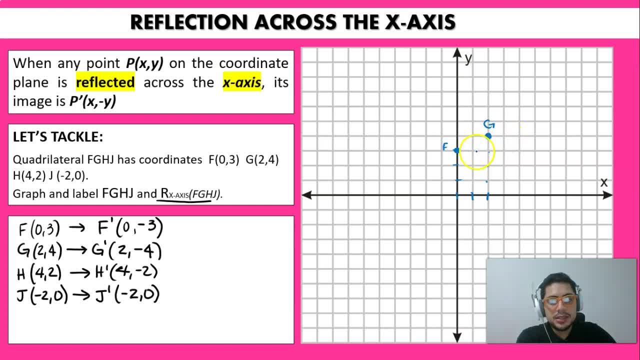 this is g, And then we're going to see that h is four comma two, So one, two, four and two, So it's going to be h here. And we're going to have that j is minus two comma zero, So one, two. So it's going to be here, And then let's just, you know. 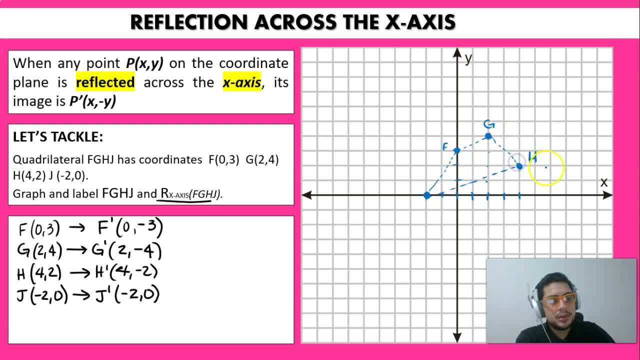 see our quadrilateral. Okay, so this is going to be our quadrilateral. So this is going to be j f g h or f g h, j, right, And now we're going to do the image. So 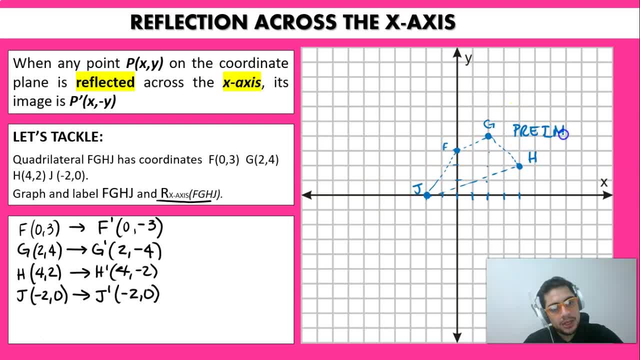 this is going to be the pre-image, or the image before the rotation, or the reflection. sorry in this case. And now let's try looking for the other image. So now the value of f tick mark is going to be zero comma one two minus three. 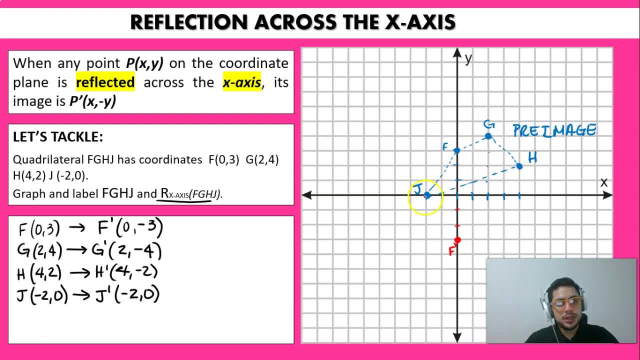 So f is going to be f tick mark is going to be here, Date tick mark is going to be on that same position right. h is going to be on four comma minus two. So it's going to be here And we're going to have that. g is going to be two comma minus four. Okay, so one, two, three. 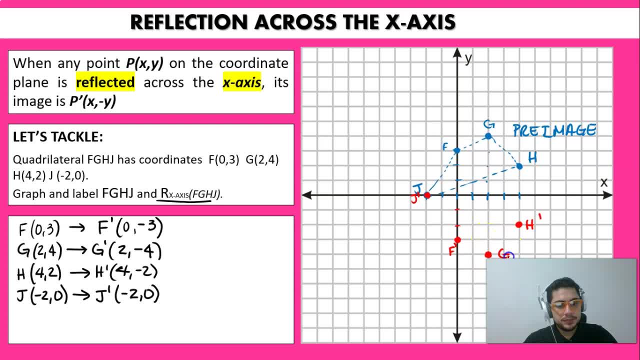 four. So it's going to be here, right, And then we're just going to see that our image is going to be like this And this is going to be our image. So, guys, this is how we find the rotated image. This is the rotation across the x-axis.